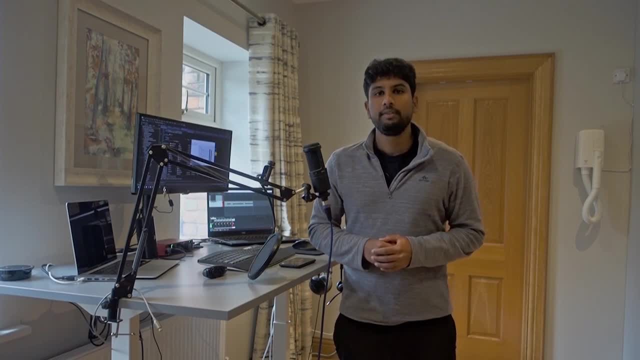 But from a distance. it doesn't have to be Intuitively. understanding these subjects, irrespective of the context, irrespective of the math, is the most surefire way of building foundational understanding and interest in the subject. So this entire series is dedicated to the discussion of one of the core areas of DSP. 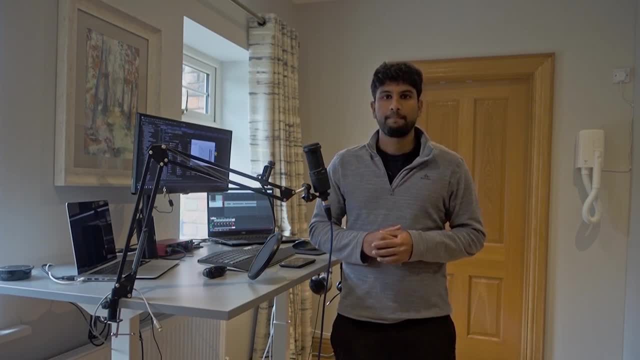 and an effect that's widely used in every realm of audio processing Filters. We'll approach filtering with as little complex mathematics as possible and rather rely on an analytical approach of simulation and visualizations to get an intimate understanding of filters, how they work. 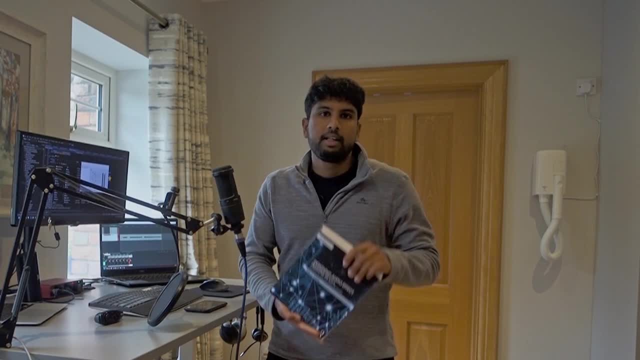 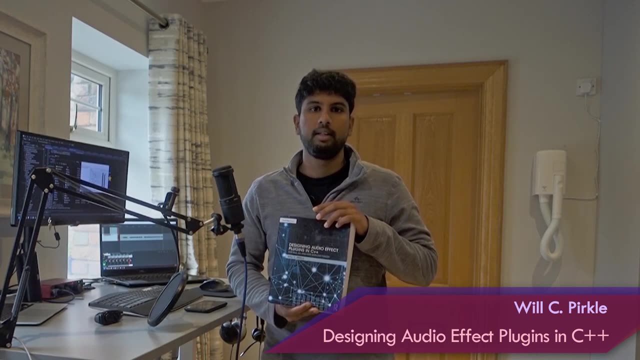 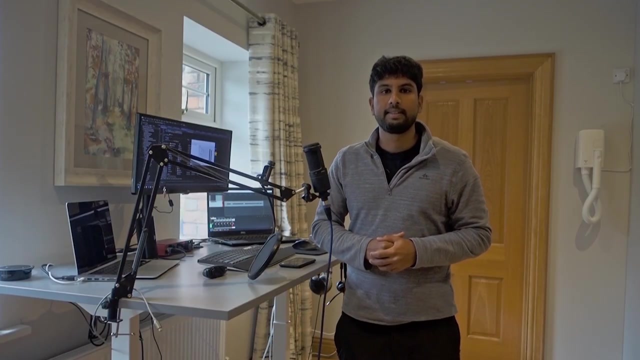 and how they behave. This section is heavily borrowed from the amazing work put together by Will Perkle in his book Designing Audio Effect Plugins in C++. If you haven't already checked it out, I encourage you to do so. So let's see what we'll be covering in this series. 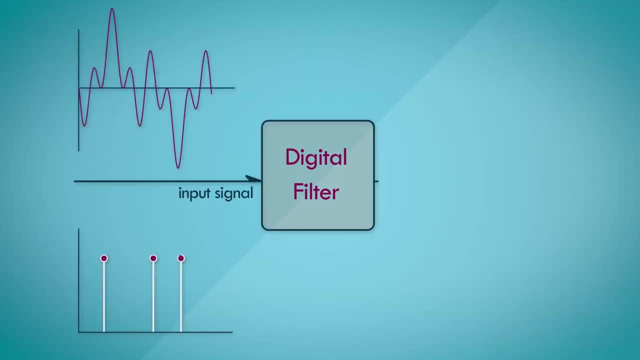 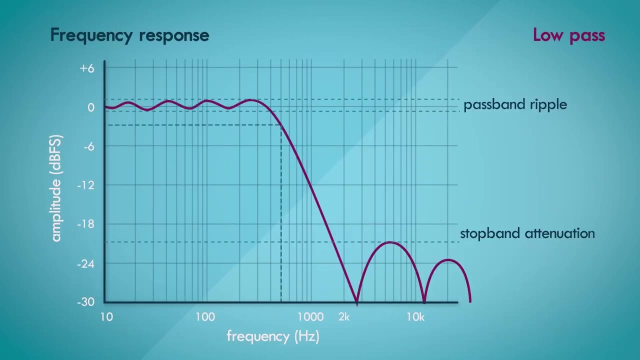 We'll start with what a filter is and the terminologies used to describe the characteristics of a filter. We'll look at a couple of ways of analyzing the result or the response of the filter by looking at the frequency and phase response graphs. 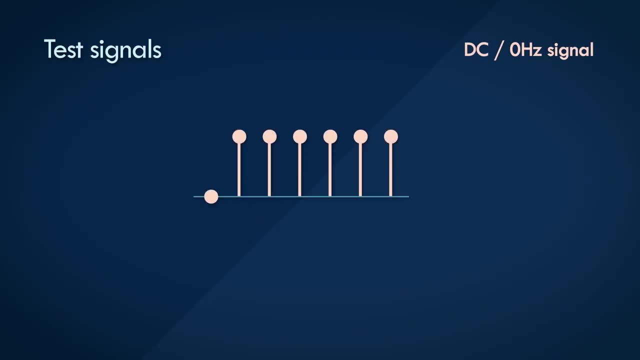 Then we'll take a quick stab at the different types of input signals that we may want to experiment with. These aren't going to be audio signals as such, but really simple test signals that we can step through sample by sample and understand how a filter might process them. 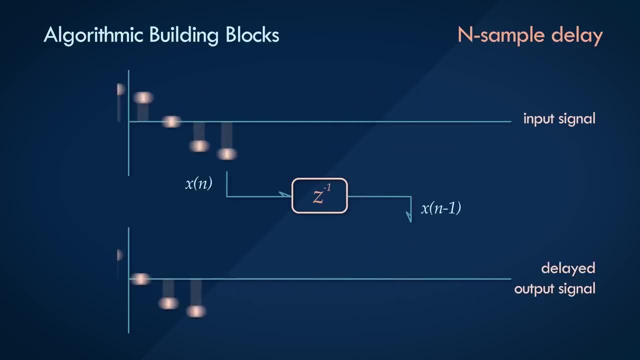 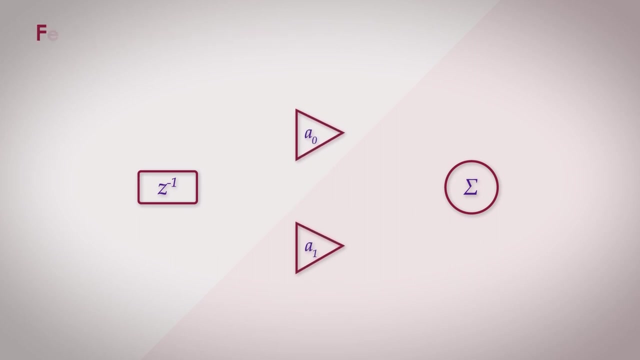 We'll look at the simple building blocks of any filter design, including delays, amps and summing mixers, and view them as structural black boxes that we can arrange in a flow diagram. We'll look at the simplest filter topology: a first-order feed-forward low-pass filter. 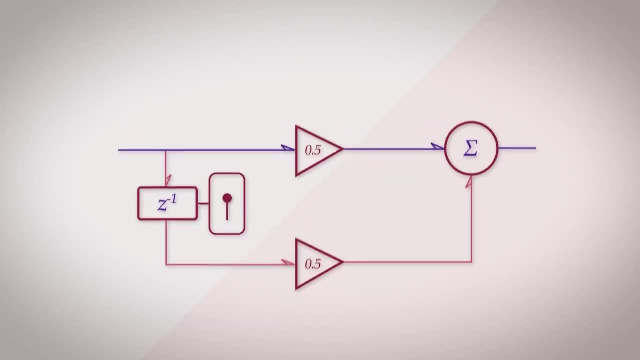 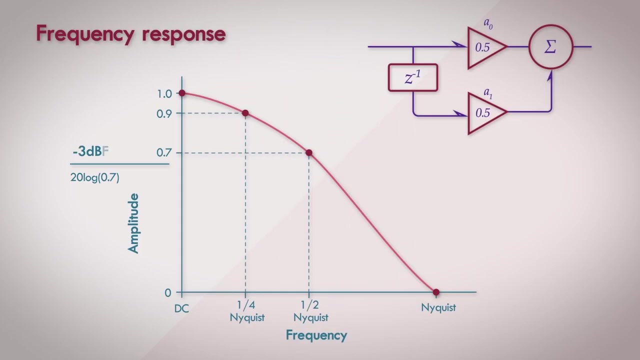 We'll run the test signals through this theoretical filter, going over the signal step by step, sample by sample, to see how the filter processes the test signal. Through this we'll discover the fundamental principle on how a filter attenuates or boosts certain frequencies in a signal. 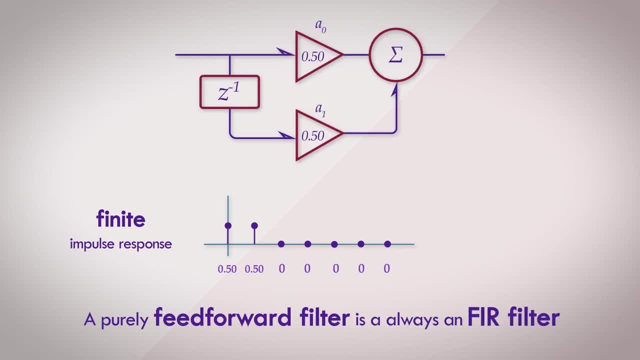 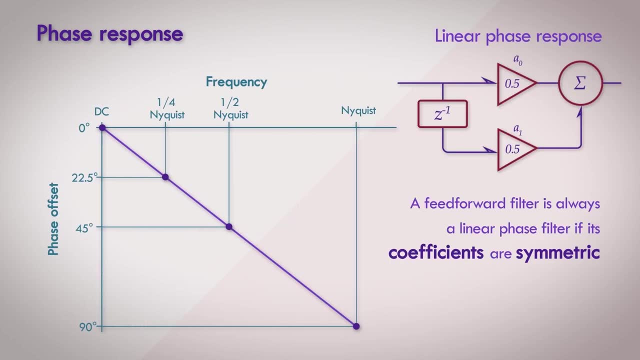 We'll look at why this filter processes the test signal. we'll look at why this filter is called a finite impulse response filter or an FIR filter, and how FIR filters can maintain linear phase characteristics. After that, we'll look at a simple modification of this topology. 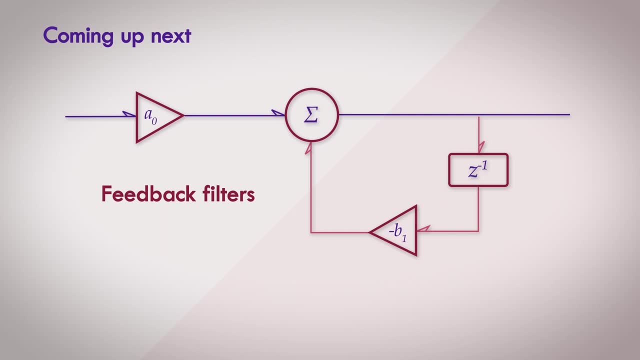 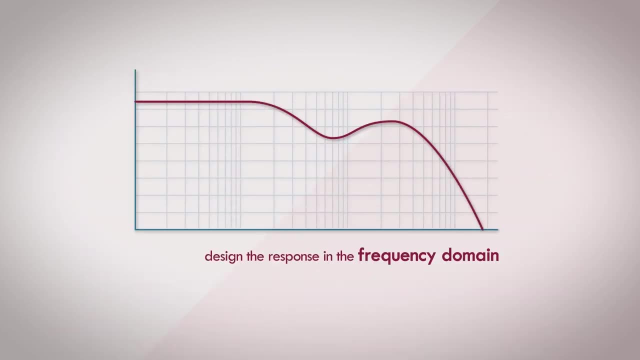 to get a first-order feedback filter and we'll do the same analysis. with this. We'll see how an introduction of a feedback loop into the topology can create a starkly different response, And we'll see why this type of filter is called an infinite impulse response filter. 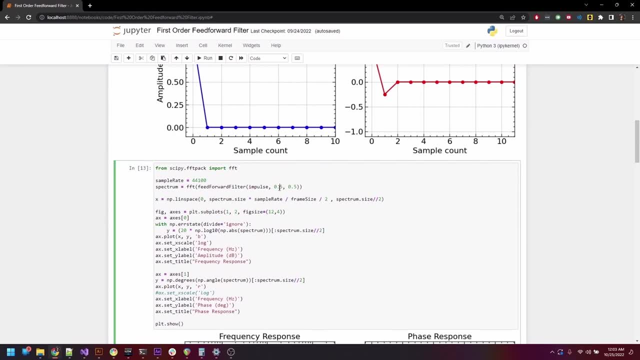 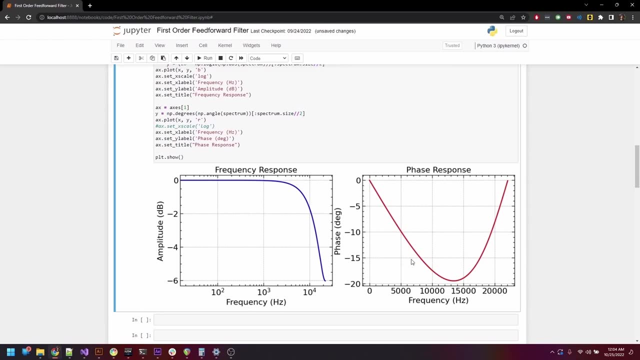 or an IIR filter. Finally, we'll take a look at a few code examples in Python which will help us solidify these concepts, and a juice plugin which implements these simple designs and try them out on some real-world audio signals. 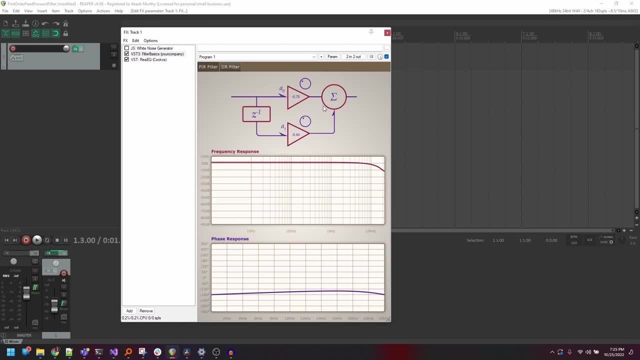 This will be a lot of fun, since we'll be building a filter algorithm in C++ with barely any mathematics at its core. Because of this, we don't use conventional filter inputs like cutoff, frequency, bandwidth or Q or gain controls. 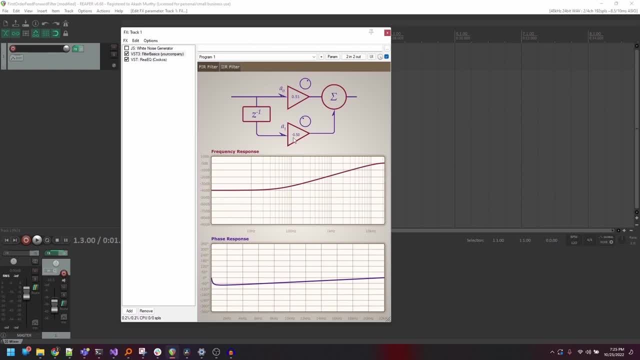 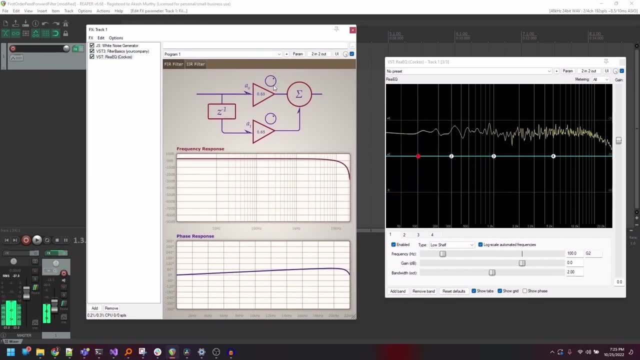 All we expose is a couple of coefficients that we can control, and it's fun to see how changing them will result in really unpredictable behavior in the filter response and ponder upon why it behaves the way it does. So with that introduction out of the way, let's get started. 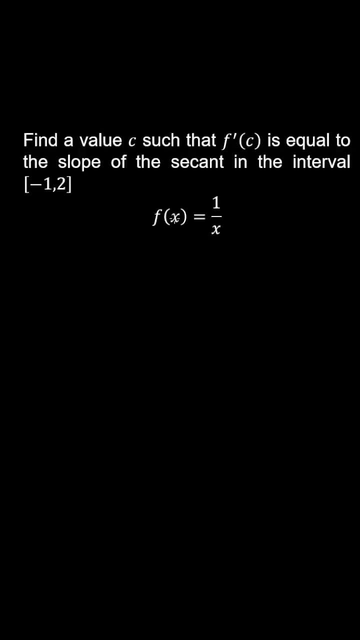 Let's find the value c such that the derivative of the function here evaluated at c is equal to the slope of the secant in this interval. While evaluating the derivative of this function at c gives minus one on c squared and we equate that with the slope of the secant. 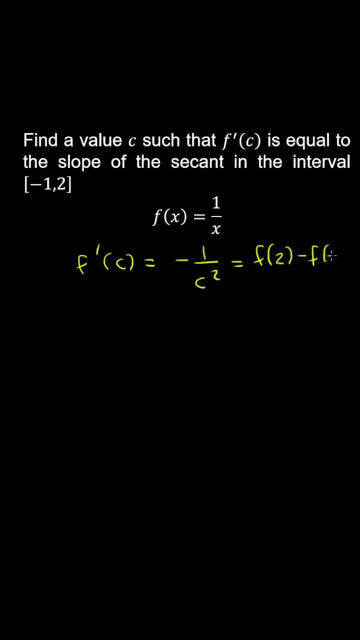 which is f of two minus f of minus one over two minus negative one by the mean value theorem. So what this gives is minus one on c squared is equal to one half minus negative one which is plus one over three. so that will be minus one on c squared. 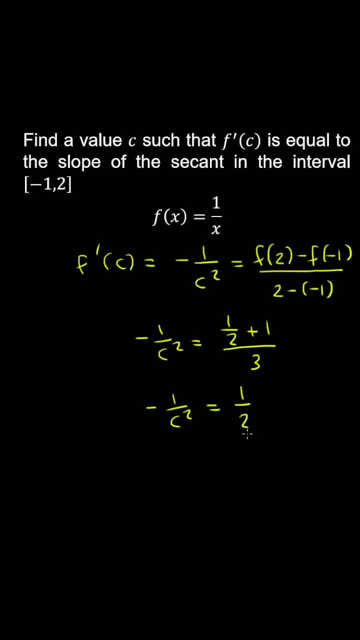 is equal to three on two on three, which is one half. So therefore c squared is equal to minus two and there's no solution to this equation, so there's no such value c in this interval where the slope of this curve is equal to the slope of the secant here on the right hand side.